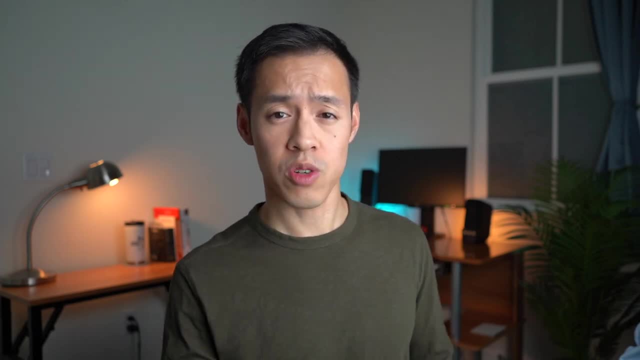 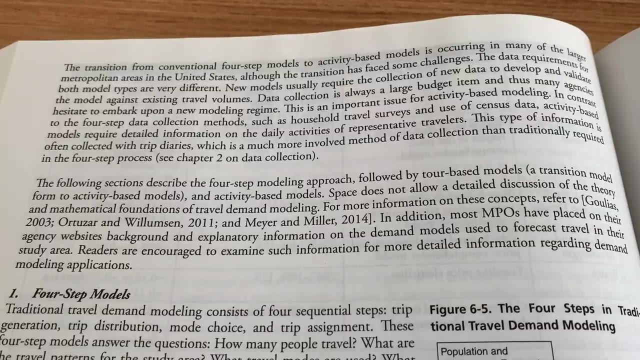 even gets designed. Here are some big ways they help shape our transportation infrastructure. In order to plan, they need to figure out where and what kind of infrastructure to build. This can involve modeling, which looks at the trips that people take from their house to their work or in other places they want to go at a regional 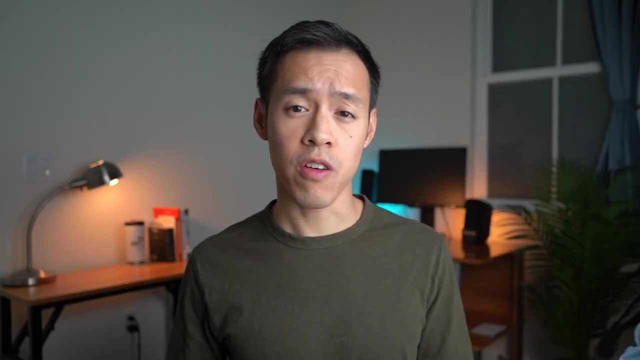 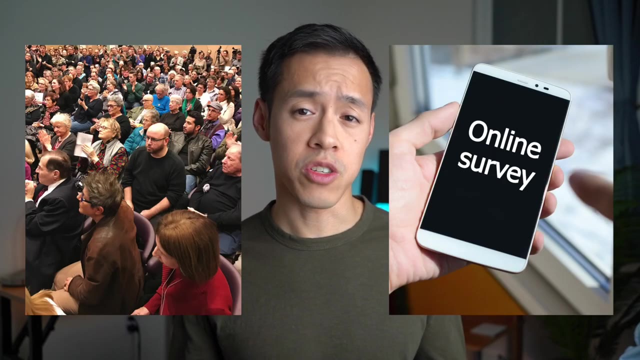 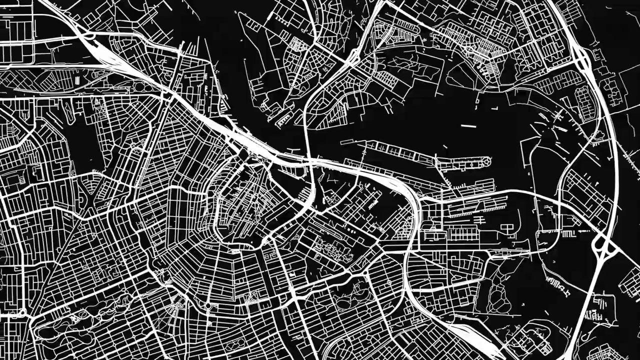 level. This involves very complex computer software and simulation. Another way they can find out is through engaging the community directly, through community meetings or, for example, outreach surveys. They also have to analyze a wide range of interdisciplinary data using geographic information systems or GIS. Through this they can see how a project relates. 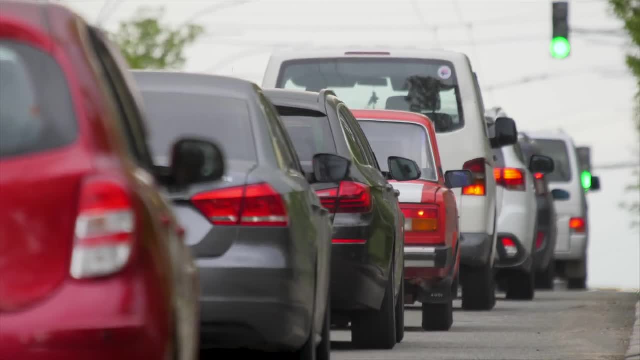 to the many different aspects of society. They also have to analyze a wide range of interdisciplinary data using geographic information systems or GIS. Through this, they can see how a project relates to the many different aspects of society. For example, they can look at environmental impact or climate change data. 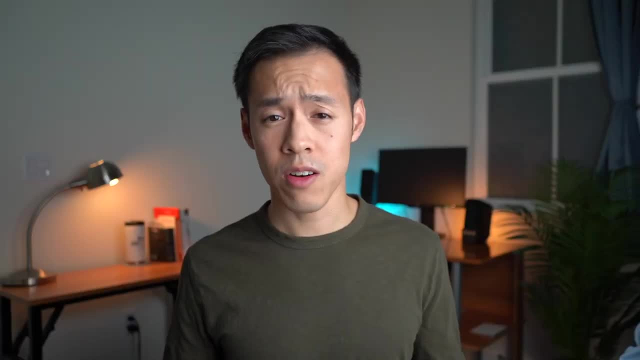 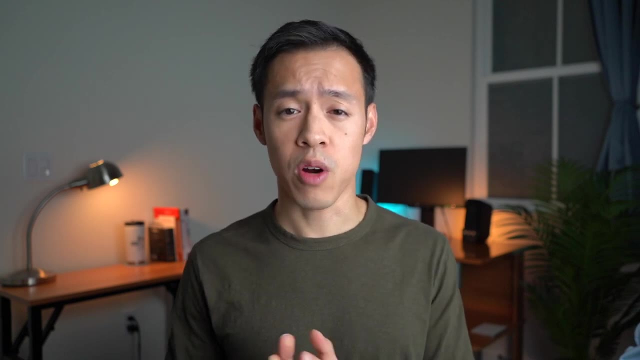 They can also look at economics and equity. Understanding how all this data relates is a key responsibility for the transportation planner. Another way planners contribute to transportation infrastructure is through the funding process. How does infrastructure get funded? There are many ways, and transportation planners often are involved with getting funding. for transportation projects. This can be done through grants, fee programs or taxes and local funds. Also, planners are involved with the policy side of transportation. They figure out how a project fits within the local, regional and state policies. This can involve land use policy. 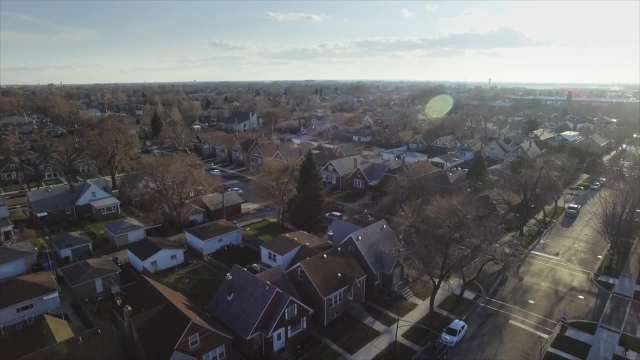 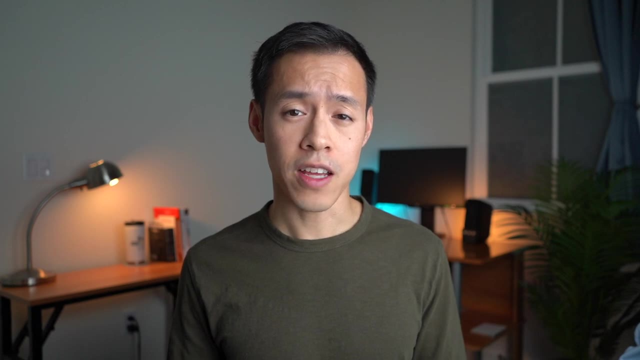 and what kind of transportation you build around that land use, or even how housing policy affects transportation use in an area. So what happens now, after the planning stage, Now that a project has been planned and the funding secured, who is responsible to designing it down to the very last? 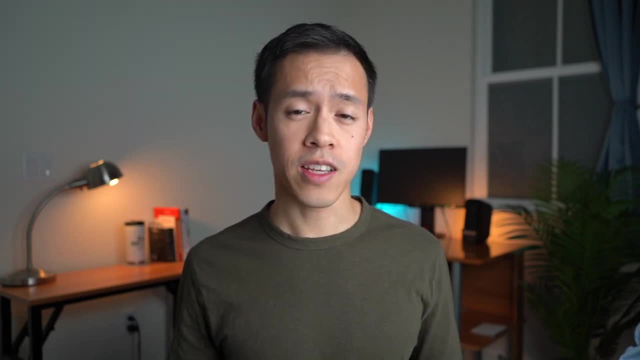 detail. That's where engineers come in. Transportation engineers focus on design and specifications of infrastructure. This is the nuts and bolts of how you build something. They do this by using advanced CAD software. In order to design something correctly, they have to follow very specific design manuals and criteria. They can also be involved with 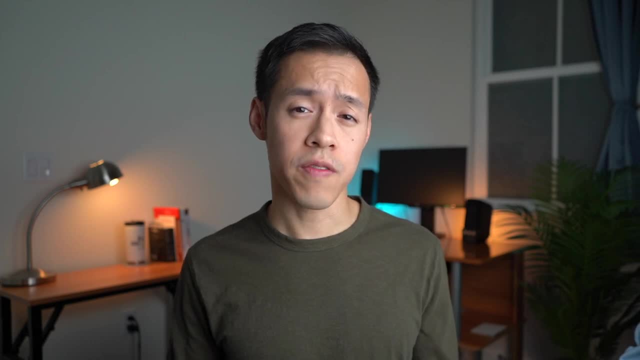 managing the construction side of the project. Things they can oversee is the construction phasing of the project to make sure that it will be built within a certain time frame, and also ensuring that the infrastructure is built according to the design and specifications of the project. After a project is built, engineers can also be involved with maintenance. 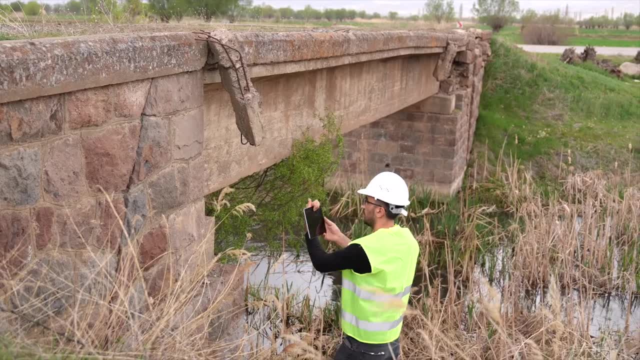 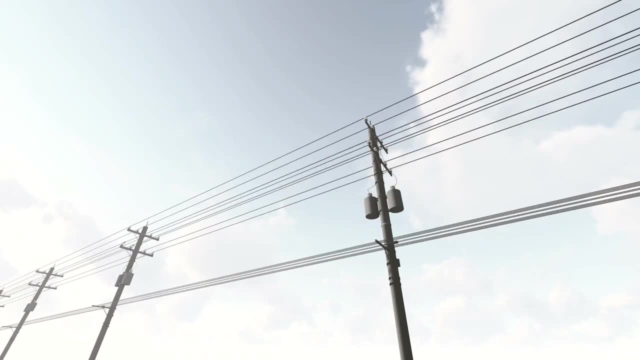 which is making sure that the infrastructure will last for a long amount of time and kept in good condition. Because of this, transportation engineers spend a lot of time dealing with technical field-related issues, For example, how to relocate utility poles to a certain design or what size of conduit to use for the wires for traffic safety. 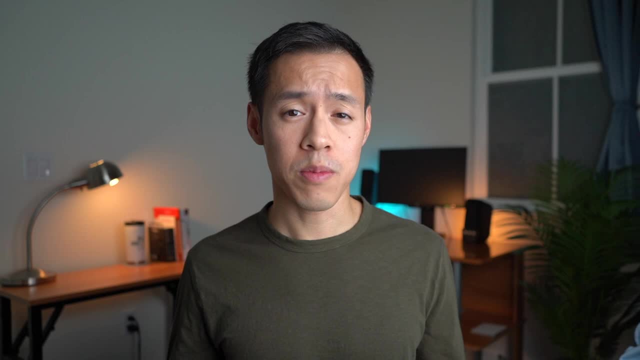 or how much aggregate base is needed for a new road. Now that we have an idea of some of the major differences between transportation planner and transportation engineer, let's talk about where they can overlap in responsibilities. It's actually common to see some of them to do key duties of the other when it's needed. Here are some of the times. 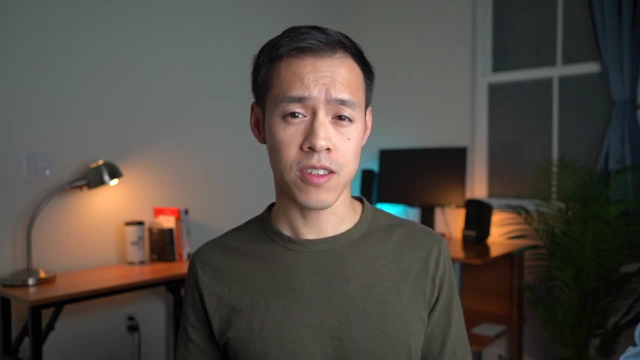 when I've seen that happen. Both are involved with transportation safety analysis, as safety is a very important part of what they both are trying to achieve, but they may differ in how they choose to analyze it and the tools that they use. Both of them are also involved with modeling. 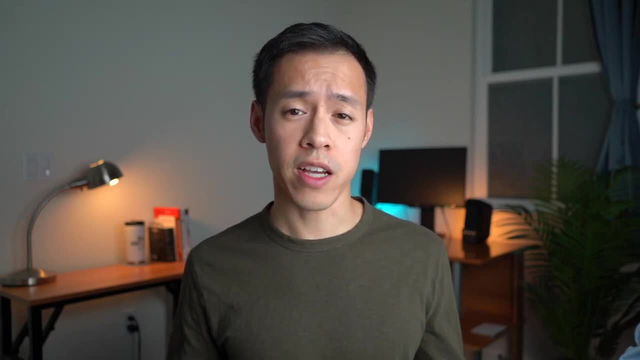 although it's mostly planners who work with large regional and very complex models, I've also seen transportation engineers use models to analyze trip generation and for local projects. In my experience, I've also seen transportation planners and engineers work on the funding side. too Many engineers work on grants alongside planners and they both can have different. 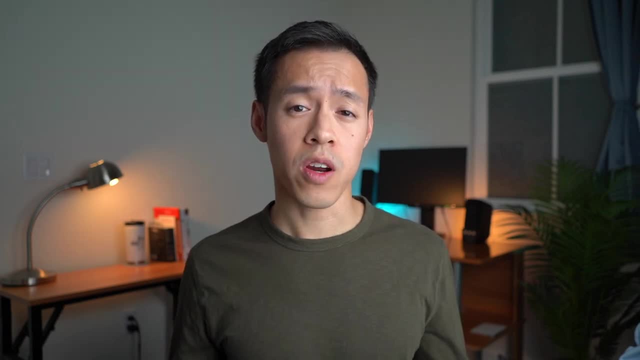 roles to fulfill in the grant application process. Lastly, I've seen both work on multimodal solutions, which means solutions for bicycle transit or pedestrians. There's a growing number of transportation professionals who are looking to improve these modes of travel, and that's really. 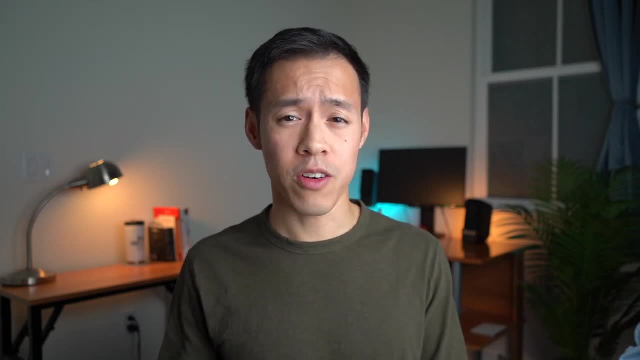 exciting to see. So now let's talk about the career paths of a transportation planner or transportation engineer. Transportation planners can come from a variety of fields, but they commonly have an urban planning background. They can also be knowledgeable about many subjects like geography, economics or even political science. Transportation engineers: 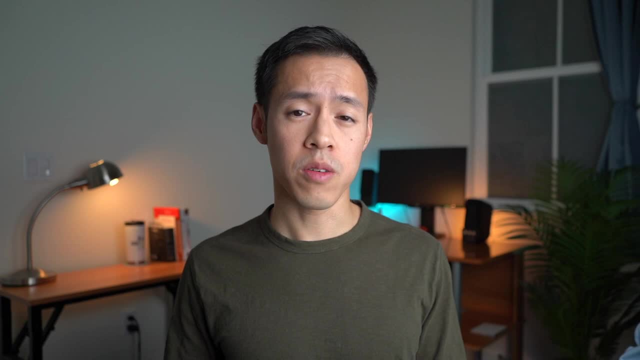 almost always have a civil engineering background. In their studies, they're required to learn multiple hard sciences like chemistry and physics, and also multiple years of calculus level math. In my experience, it's actually possible to do both transportation engineering and planning, but there are some things you should know about. Many engineers I know today are involved with the. 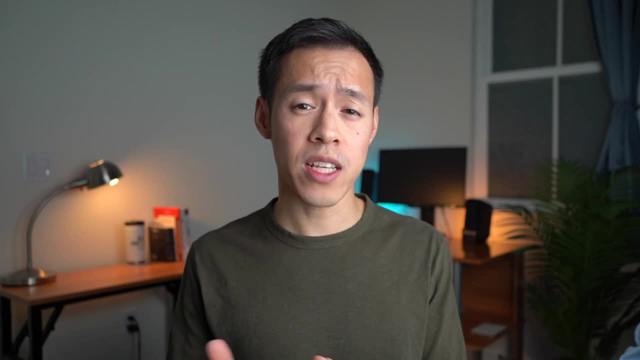 transportation planning process in some form, or have even transitioned to do transportation planning duties on a daily basis. And in my opinion it's actually easier to do this than the other way around, because in the earlier parts of your career it makes sense to focus on the 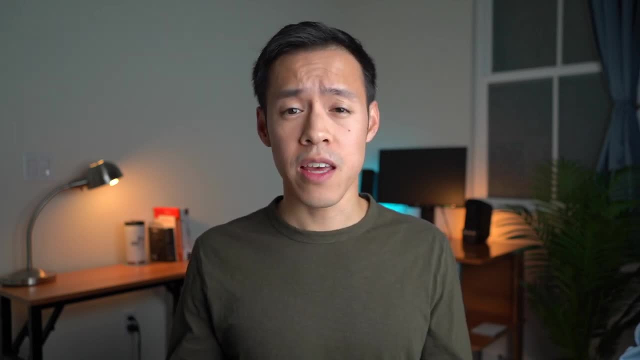 details of design and things. But then when you get more experience and you move up, you tend to start managing more larger, more complex and more complex projects. So I think it's important to think about the big picture, which is actually more transportation planning.